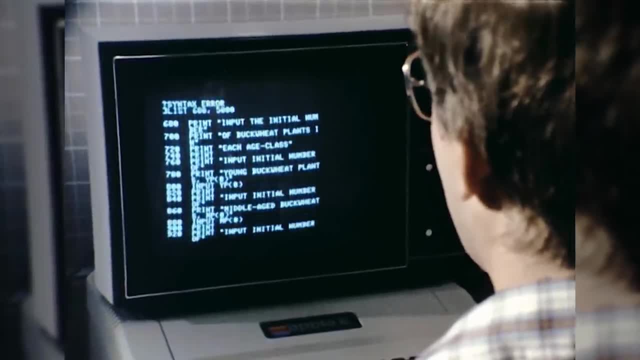 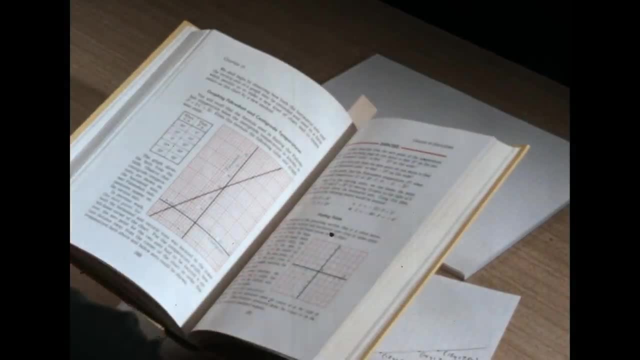 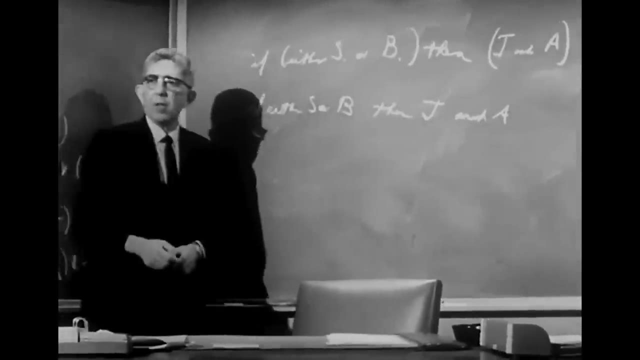 I was doing anything scientific until after I had published enough papers that it finally occurred to me My education was as a mathematician. It was just natural for me to think about computers as a mathematician. When you write an algorithm, you need to have a proof that it's correct. An 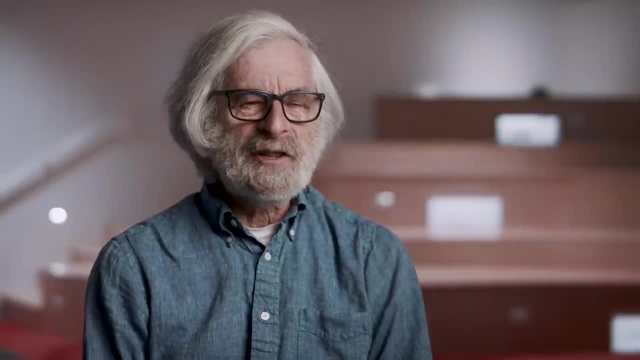 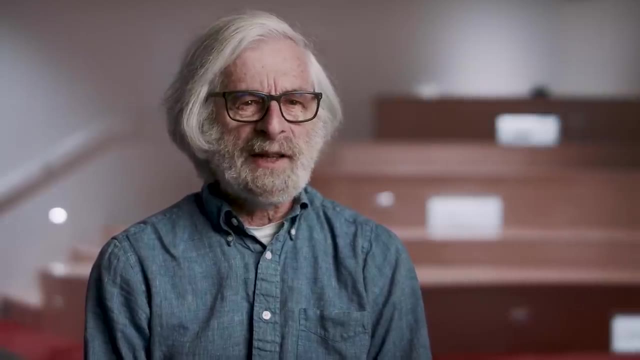 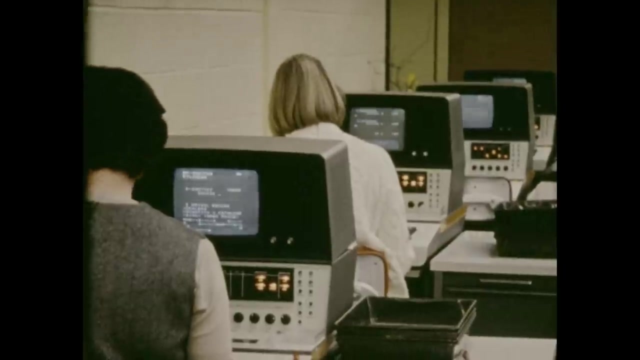 algorithm without a proof is a conjecture, It's not a theorem, And if you're proving things well, that means mathematics. Computer scientists tend to think in terms of programming languages. One of the epiphanies in my career was the realization that I was not writing programs, as 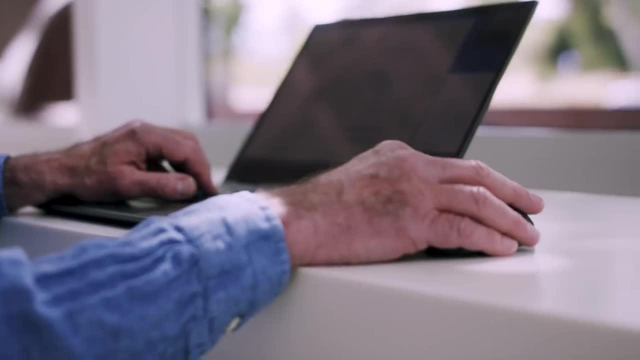 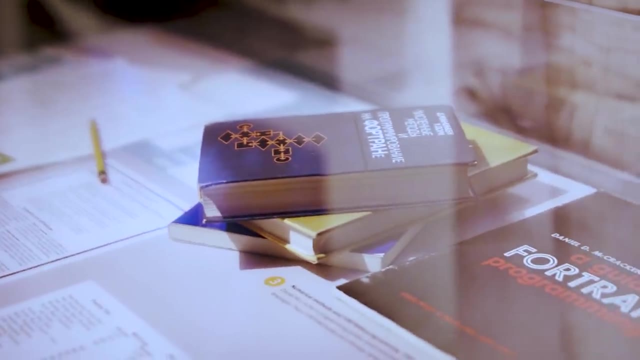 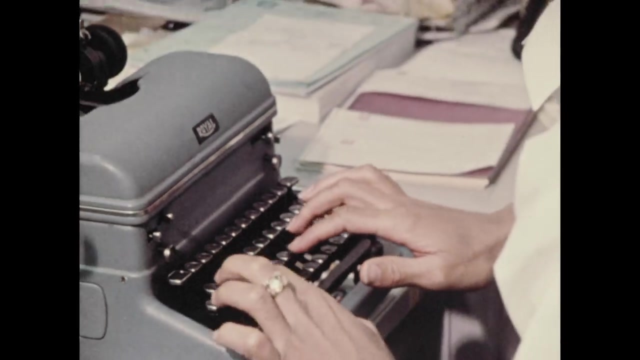 a computer scientist. I was designing algorithms. I came to realize that if I'm not writing a program, I shouldn't use a programming language. People confuse programming with coding. Coding is to programming, what typing is to writing. Writing is something that involves mental effort. You're 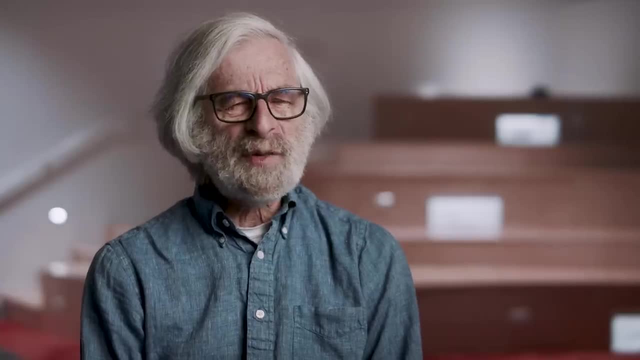 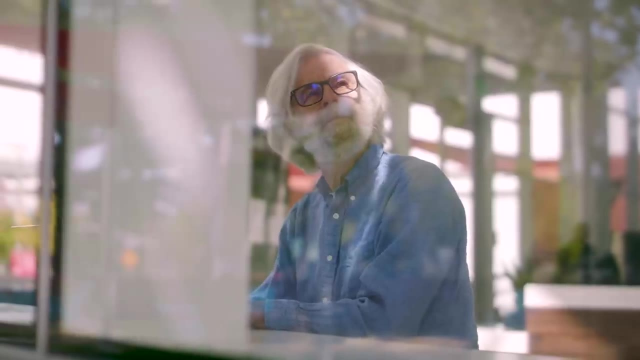 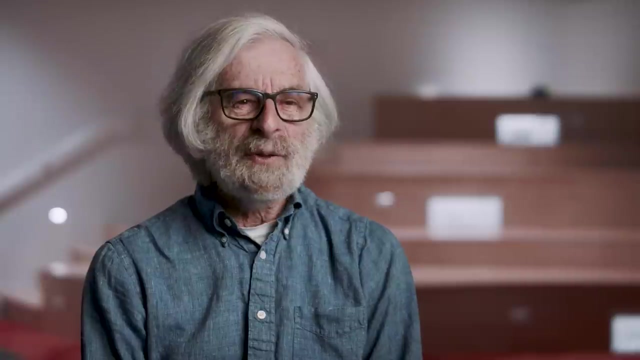 thinking about what you're going to say. The words have some importance, but in some sense, even they are secondary to the ideas. In the same way, programs are built on ideas. They have to do something, And what they're supposed to do, I mean, is like what writing is supposed to convey. 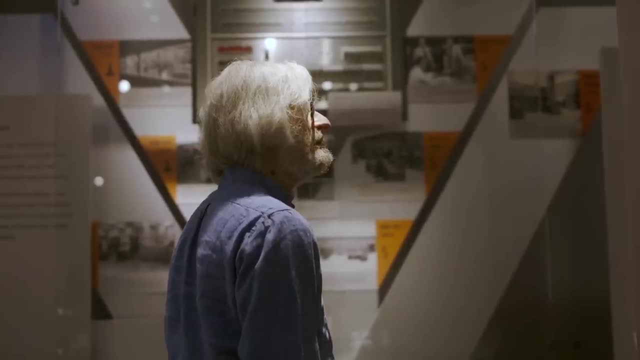 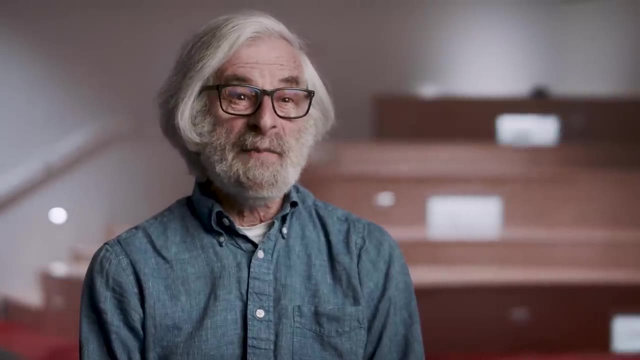 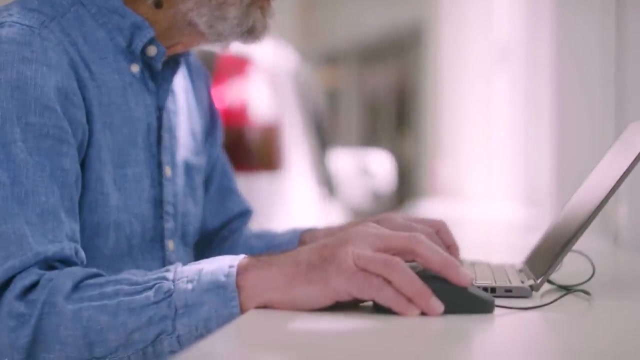 If people are trying to learn programming by being taught to code, well they're. They're being taught writing by being taught how to type, and that doesn't make much sense. The best way I have for teaching about programming as distinct from coding is to think about. 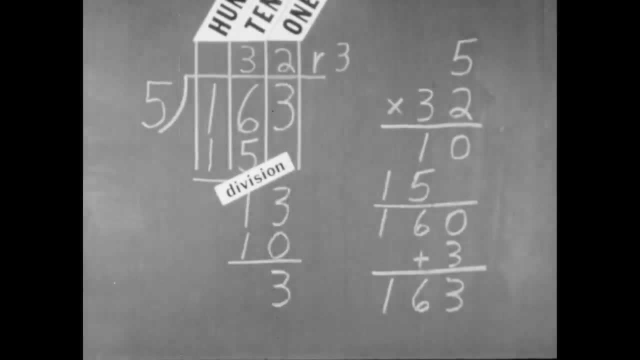 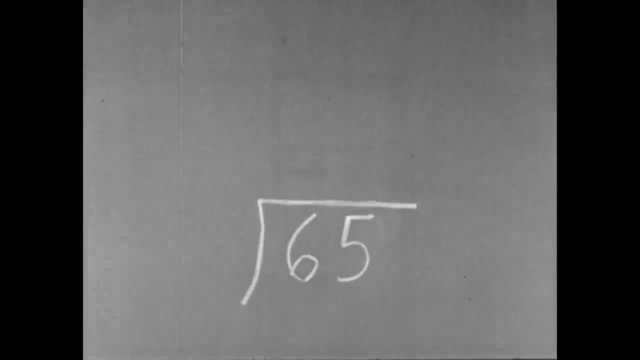 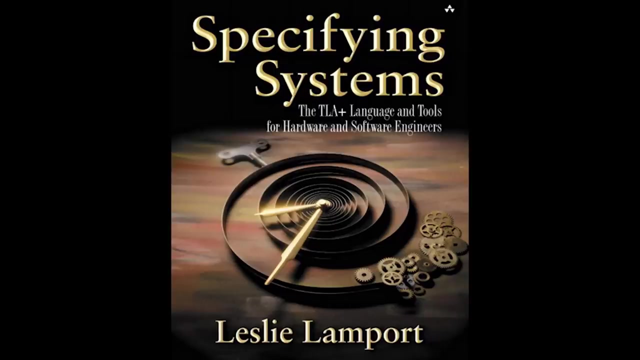 what the program is supposed to do mathematically. There's a very big practical problem with this. The mathematical education in this country is pretty terrible. Most people wind up being afraid of mathematics. This is even senior programmers. I've developed a language called TLA Plus for writing down the ideas that go into the 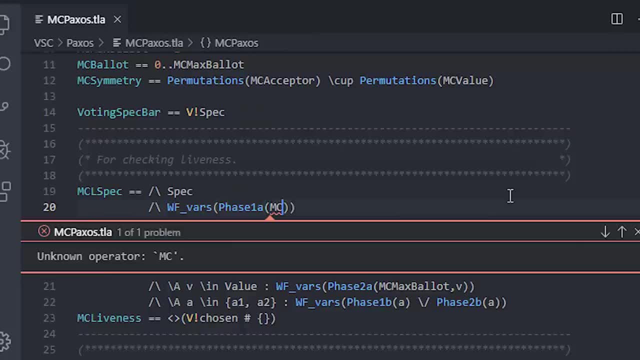 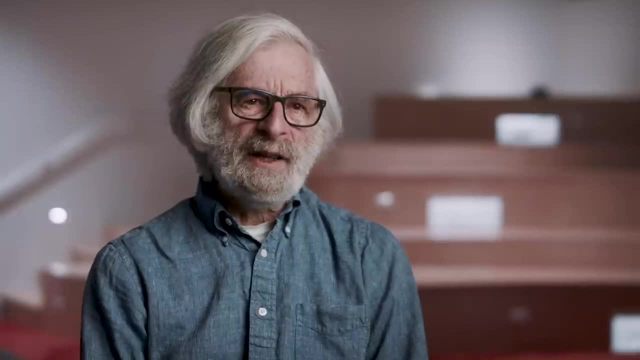 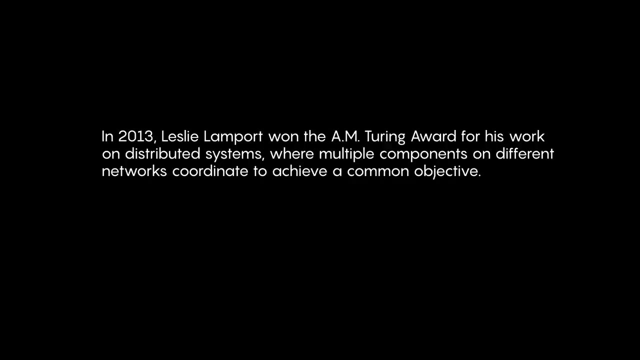 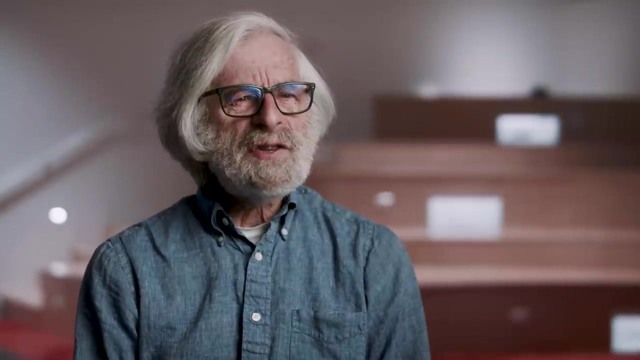 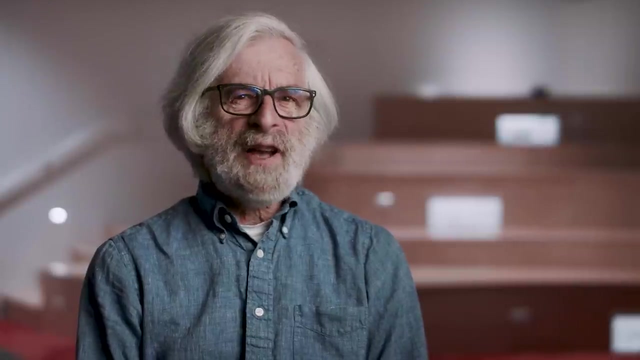 program before you do any coding. It's a pretty hard thing for engineers to get into, but when they do, it develops their ability to think mathematically. A distributed system is one in which your computer can be rendered useless by the failure of a computer that you didn't even know existed. 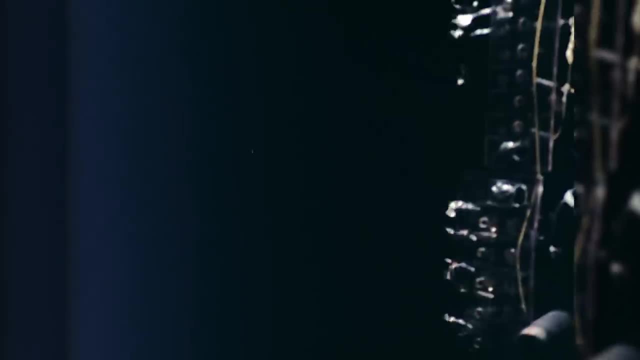 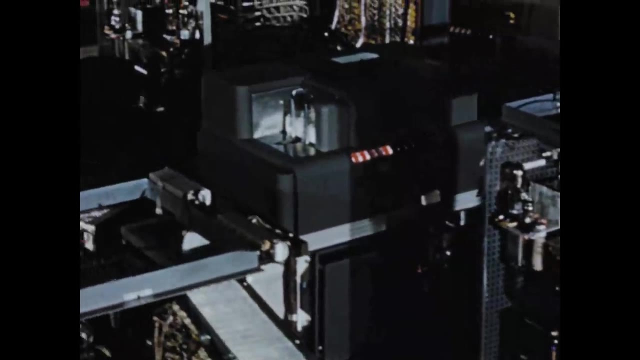 Non-distributed computing is when different processes communicate by using the same memory, and distributed computing means that they're communicating with one another by sending messages. Now, my interest in computing is that I want to be a computer scientist. I want to be a computer scientist. 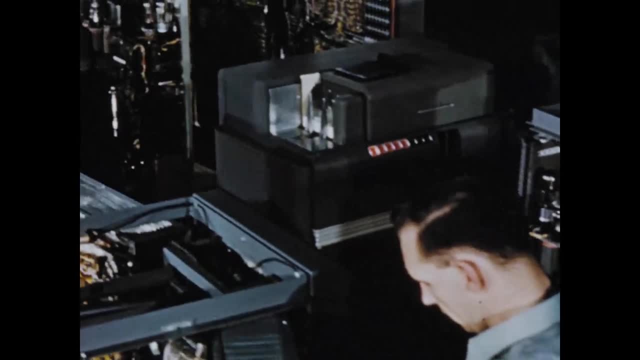 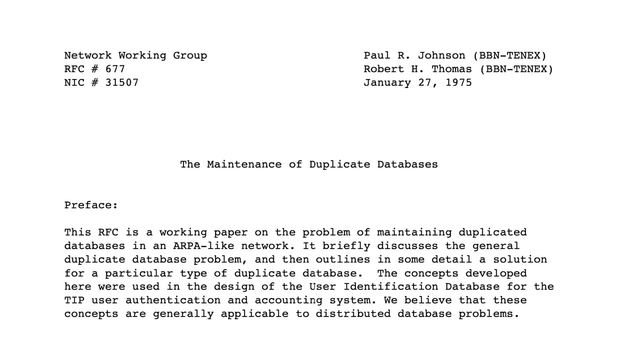 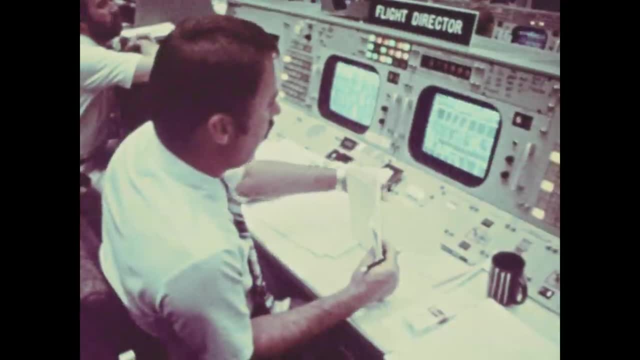 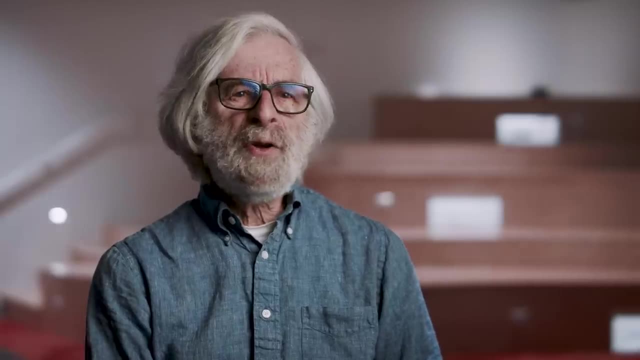 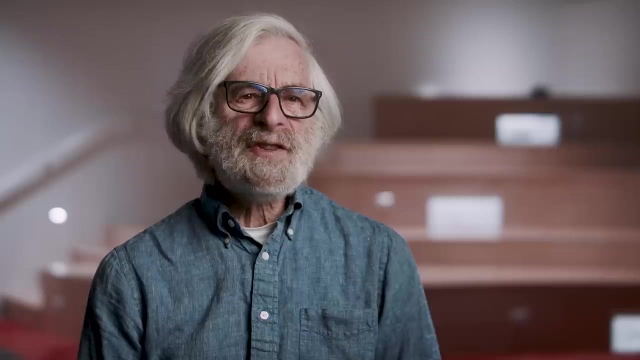 for implementing distributed databases. These are databases where you could have multiple copies of the data sitting at different computers so that programs on each computer could have rapid access to the data. but they had to be synchronized so that processes on all the computers could be synchronized. 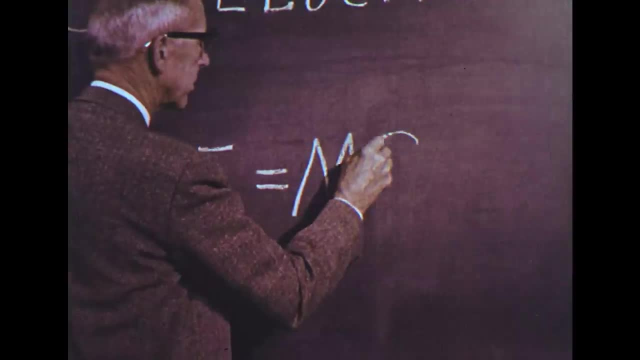 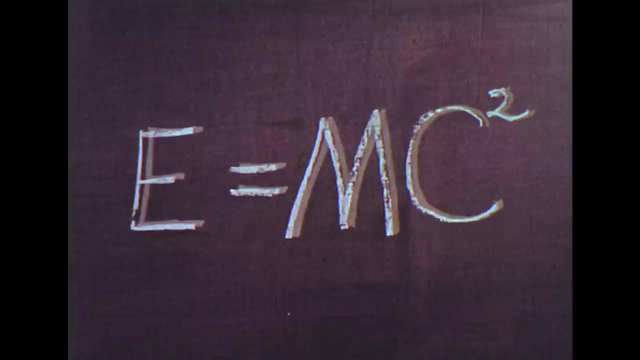 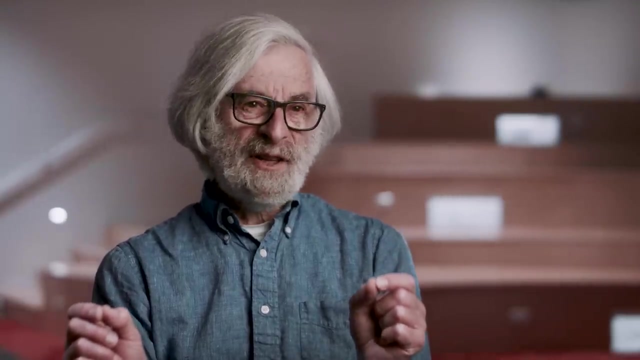 I guess it's a little false but it links you to Daniel right. ELLER CASEY, I think we want to find out something about how surveillance data is different. in Jurassic Rapids, The previous student from Dr好像 organic science, My friend Dr Adolf 86, took from a study that was out at the farther end of the ocean. 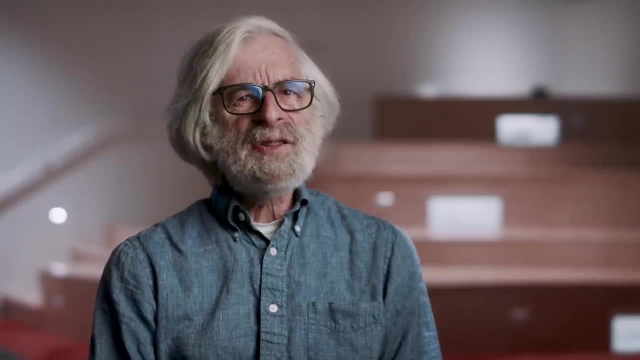 in Sierra Leone, ex interfere in the ocean emissions. scientists have come to learn one thing. What he found in his study whichplant to have Ghys Schonstein, was that the levels of activity in a region that doesn't correspond to look like the Earth's surface is the tenains. 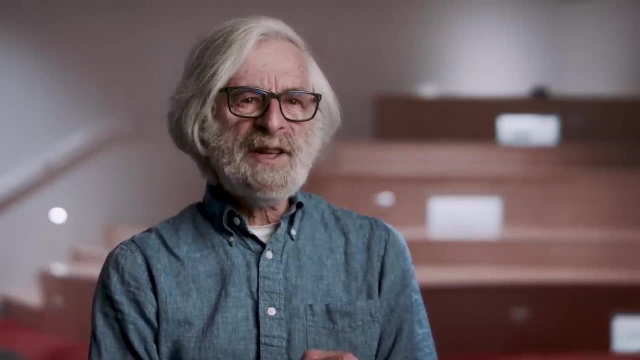 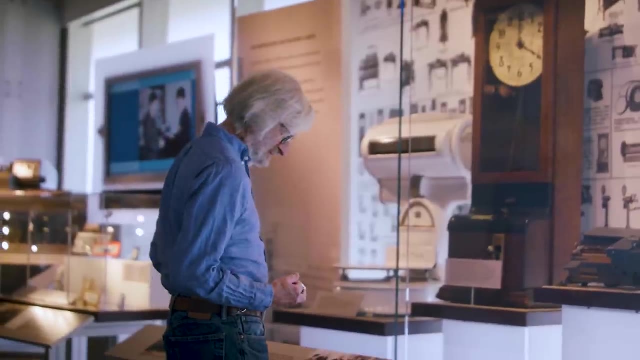 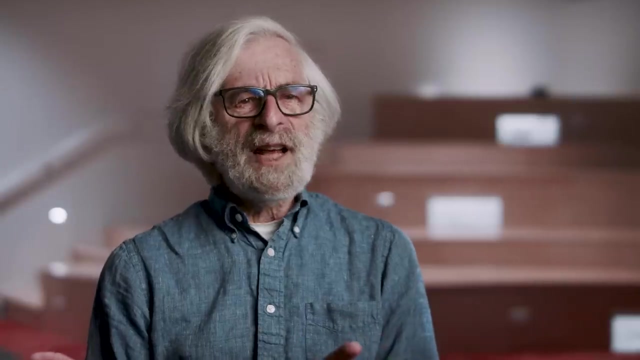 of nuclear weapons be transmitted from one event to the other when the information cannot travel faster than the speed of light. I realized that that notion of causality was violated by the algorithm of Thomas and Johnson. It's completely analogous to the relation in special relativity. 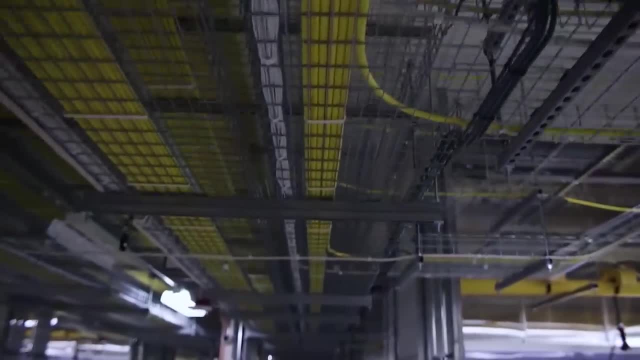 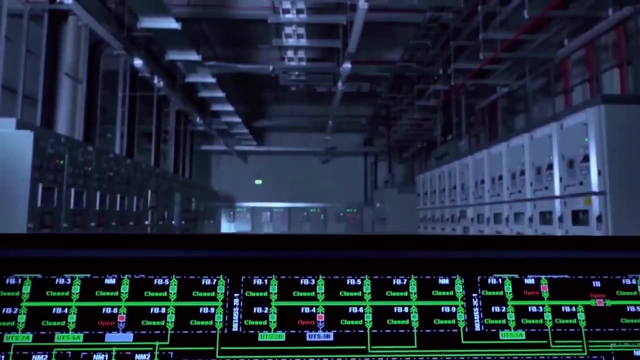 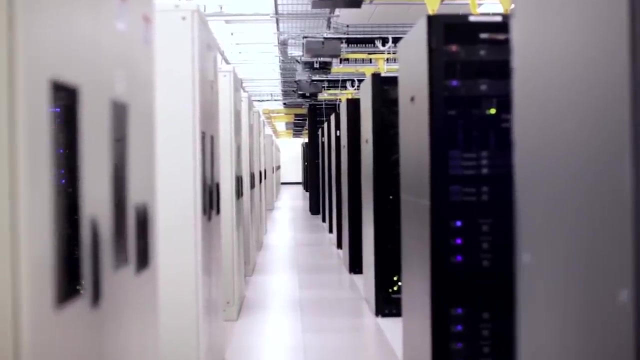 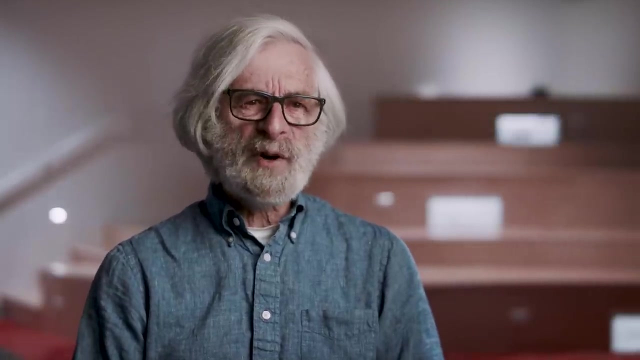 So what I did is I wrote a paper that explained this notion of causality. One could solve any distributed system problem by building what I called a state machine. Think of it as an abstract computer that does one thing at a time. You make sure that all the computers in this distributed system cooperate to implement. 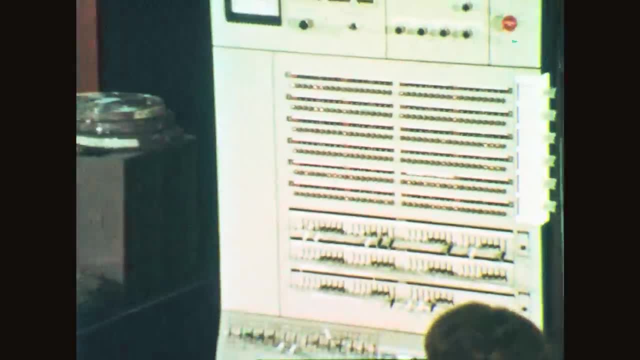 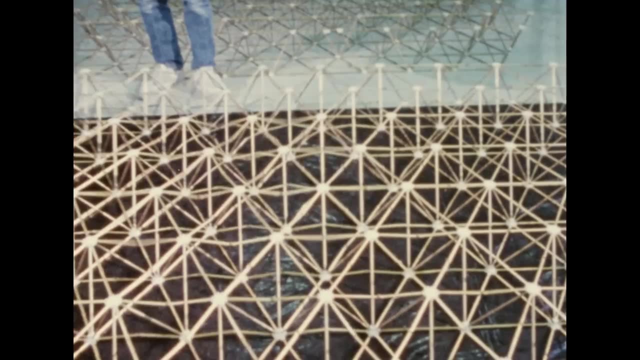 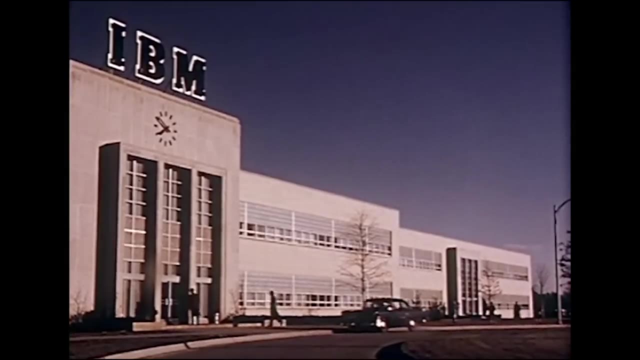 a single state machine, And that idea has become fundamental in the way people think about building distributed systems. I had never even thought about a distributed system before I wrote that paper. As I progressed in my career, I came to appreciate the idea of working in industry. 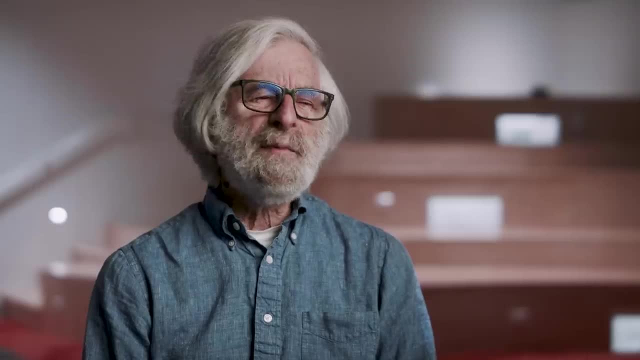 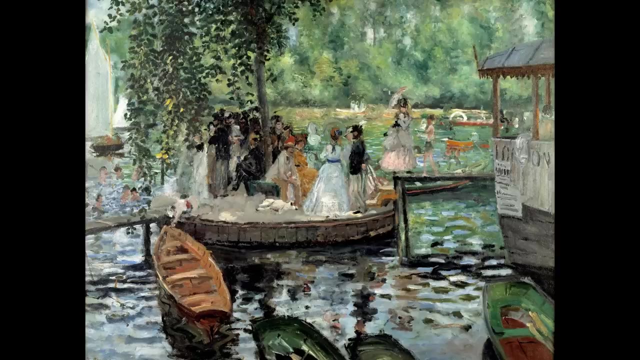 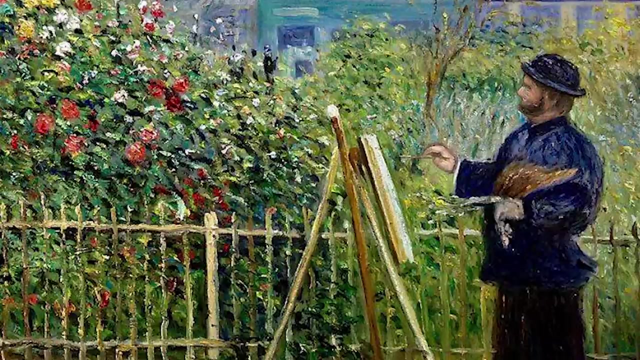 That's where most of the interesting problems that I found came from, From engineers having a problem to solve. It reminds me, actually, of something that Auguste Renoir once said. Someone asked him why he painted outside rather than in his studio, And what he said is: if I were painting in the studio and I wanted to paint a leaf, 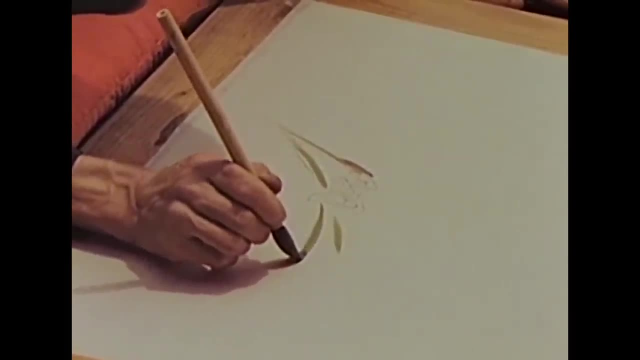 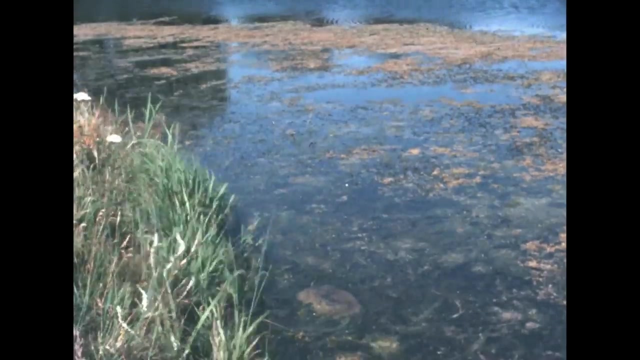 I would be able to think of only a half dozen or so different kinds of leaves that I could paint, But when I was painting outdoors, there were just these millions of different kinds of leaves that were there that I could paint from. I found my research the same way. 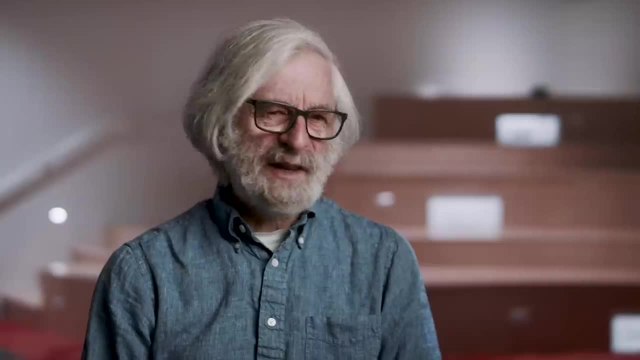 That if I sat down and just contemplated my navel and think about problems, there was a small number of problems that I could paint. I found my research the same way: That if I sat down and just contemplated my navel and think about problems, 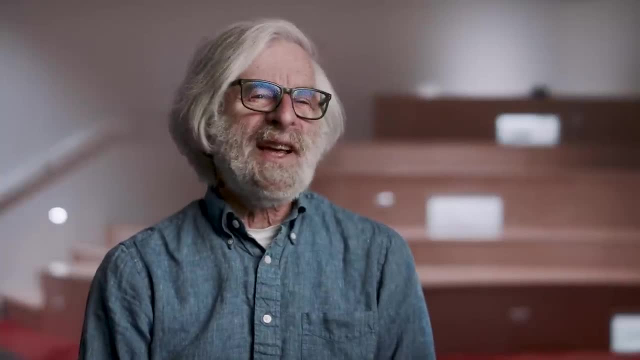 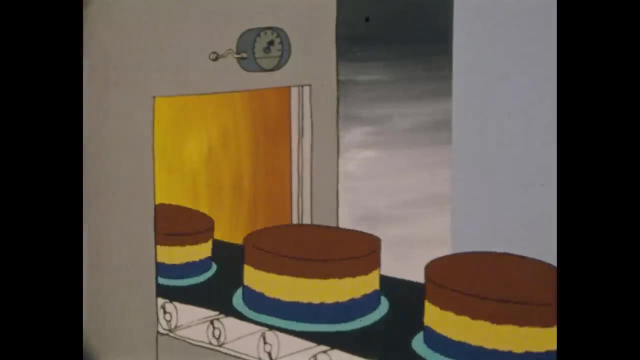 there was a small number of problems that I could paint from, But there were just scores of them sitting out in industry waiting to be solved. But there were just scores of them sitting out in industry waiting to be solved. My favorite of my algorithms is the Bakery Algorithm. 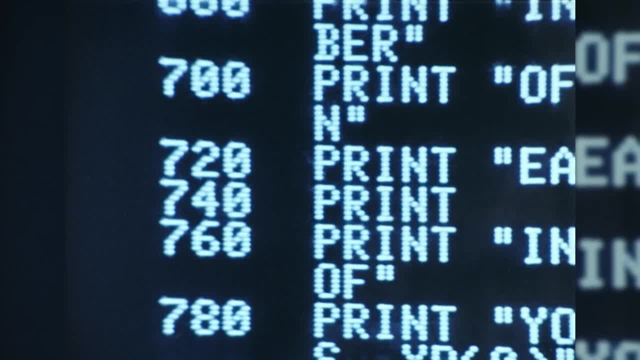 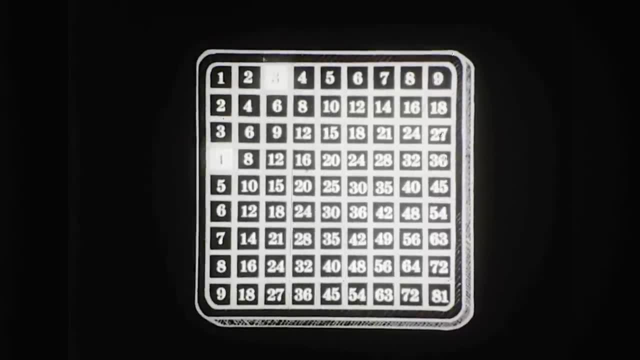 It's to solve the mutual exclusion problem, that is, keep two processes from using the printer at the same time. Processes choose a number based on the numbers that have been chosen by other processes and use an algorithm so that the lowest is allowed to use the printer.